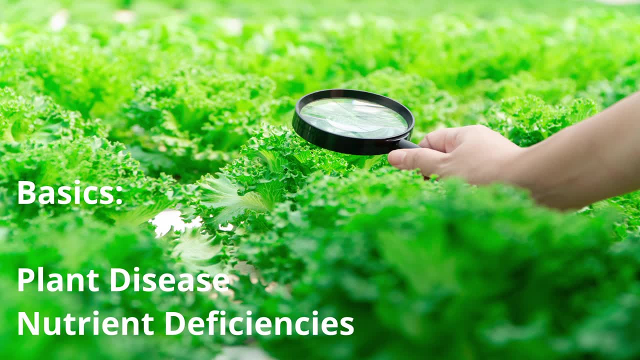 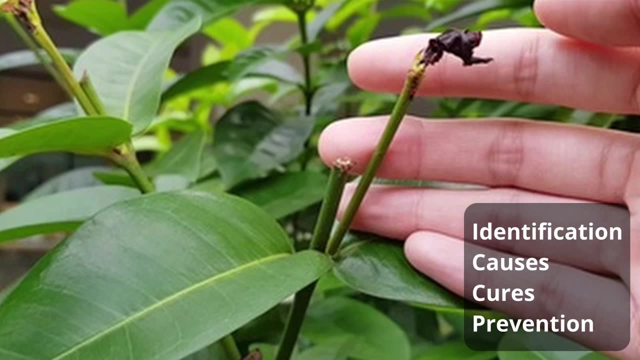 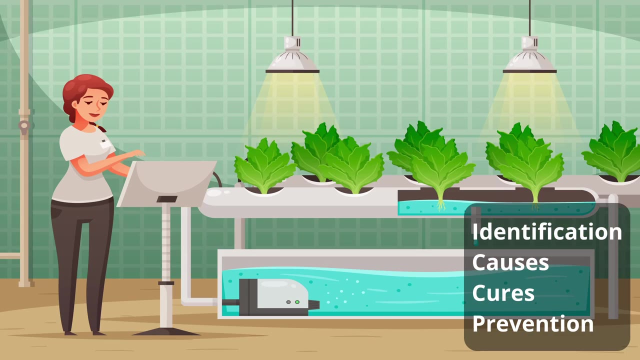 Hello everyone. In this video I will go over the basics of nutrient deficiencies and plant disease. We will review how to identify the problems, with examples and causes, cures and prevention. This is a short video intended for the beginner gardener or, like me, an amateur hydroponic enthusiast. 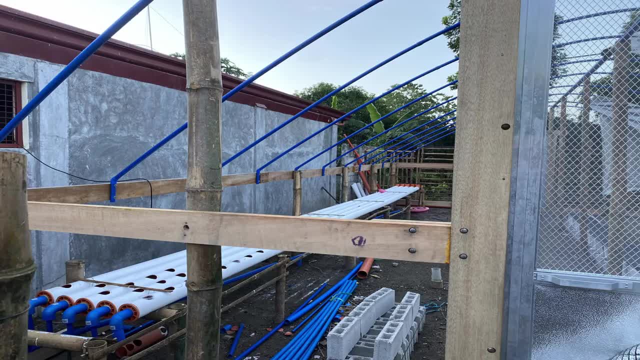 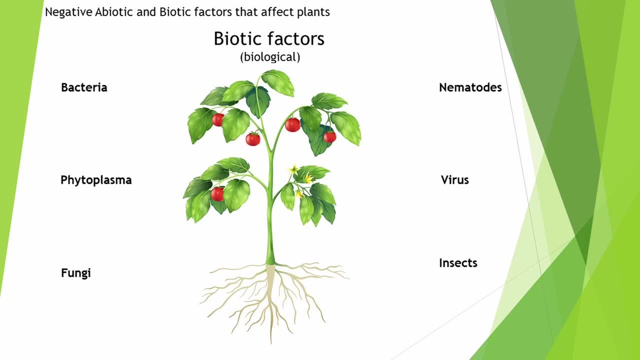 Welcome to Expat Hydroponics. Problems with plants are separated into abiotic and biotic factors. Biotic are biological factors such as diseases. Examples are bacterial virus and fungal. Abiotic are non-biological factors like environmental stress and nutrient deficiencies. Just like with humans, abiotic factors 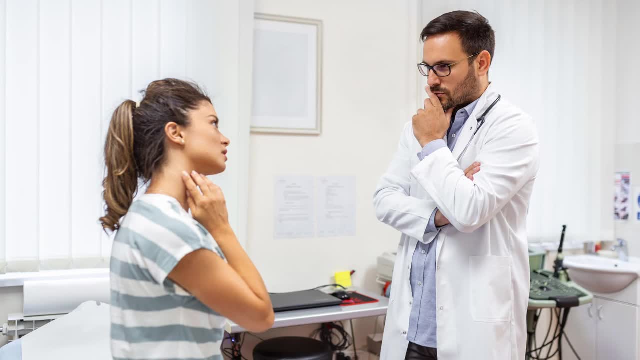 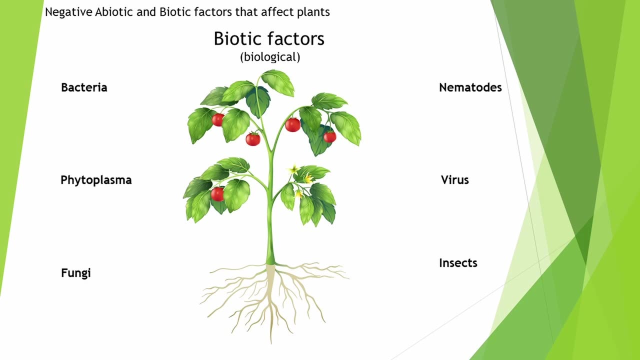 in plants can lead to biotic problems. Stress and nutrient deficiencies weaken the plants and make them more susceptible to getting sick. First, let us discuss biotic factors. Most biotic factors come from the soil and or transmitted by insects. Bacteria is the first biotic factor. They are single-cell. 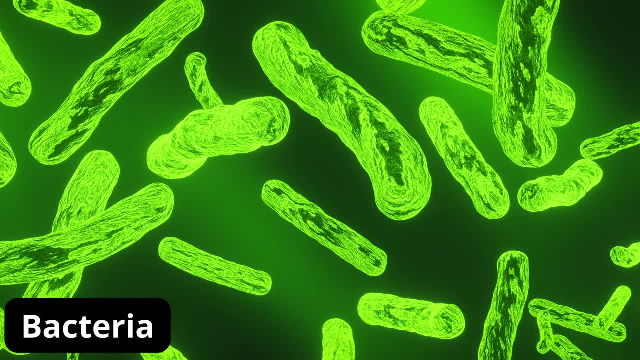 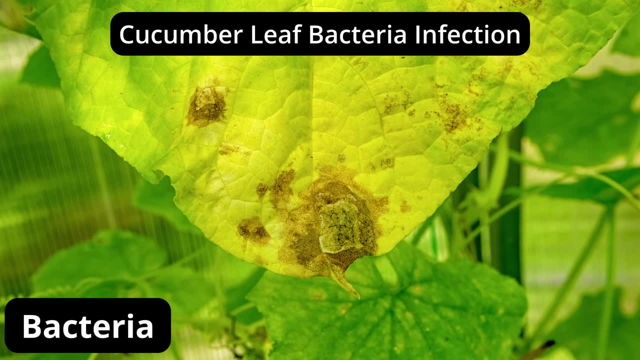 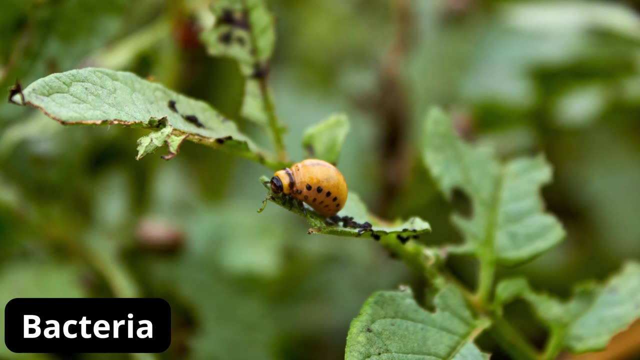 organisms and most do no harm to plants, But about a hundred species can cause plant disease, like blights, leaf spots, fruit rot and wilting. Bacteria can enter healthy plants through natural openings or wounds caused by environmental or insect damage. In a greenhouse setting, humans can also. 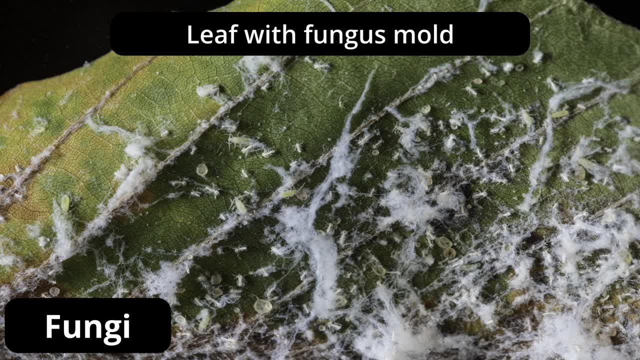 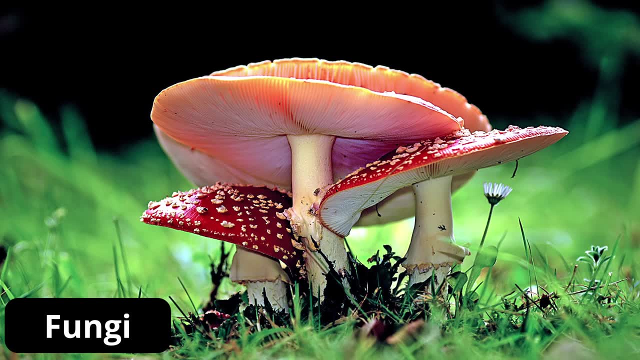 transmit plant harmful bacteria. Fungi is the next factor and usually grows as threads or strands called hyphae. Mushrooms are famously a type of fungi and not a plant. Fungi can survive in soil as spores for many years and can be. 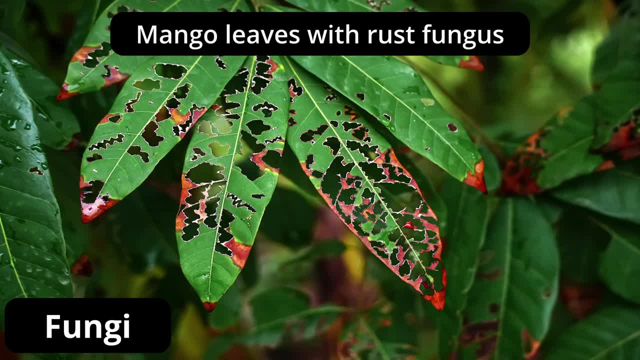 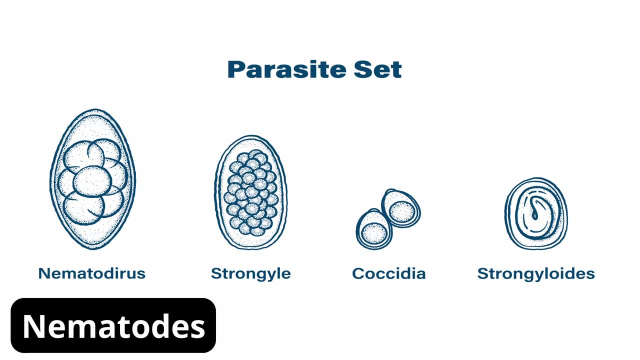 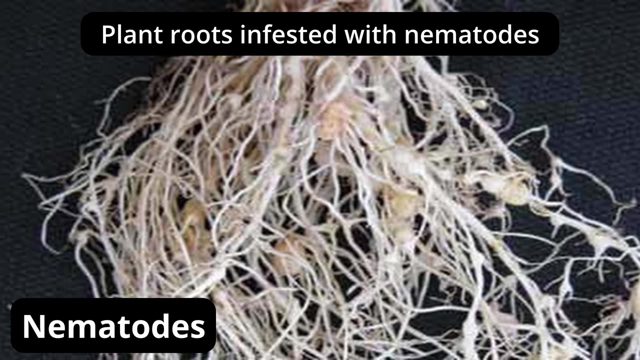 both water and airborne Fungi can cause root and stem rots, leaf blights and leaf spots, as well as vascular wilts. Nematodes, the third biotic factor, are tiny microscopic ground worms that originate in soil Feeding on the plant. they either kill the plant or damage it by reducing the 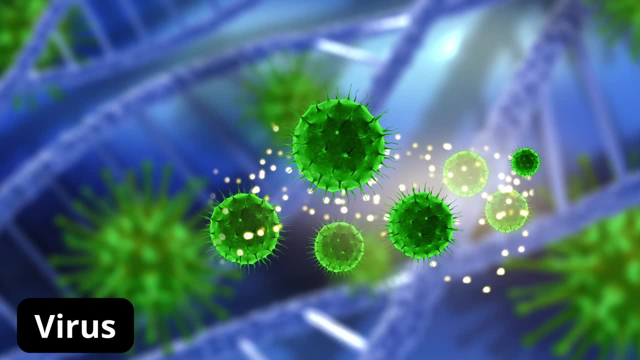 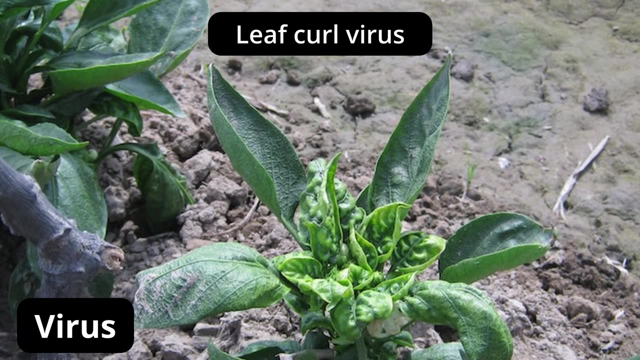 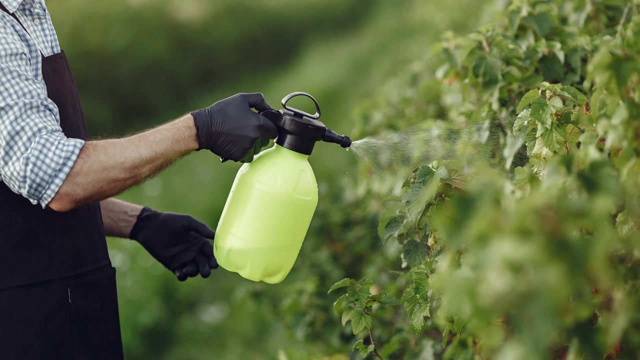 plant's ability to feed on water and nutrients. The last biotic we cover is virus. It can enter the plant via insects or nematodes and once in they multiply, causing plant stunning and mosaic or ring spores. The virus is frequently invited into the plant, forming small spot patterns on 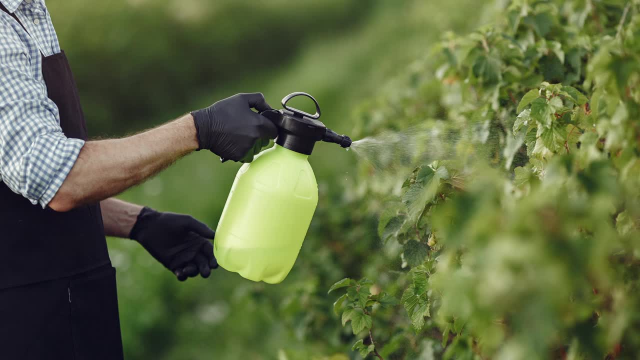 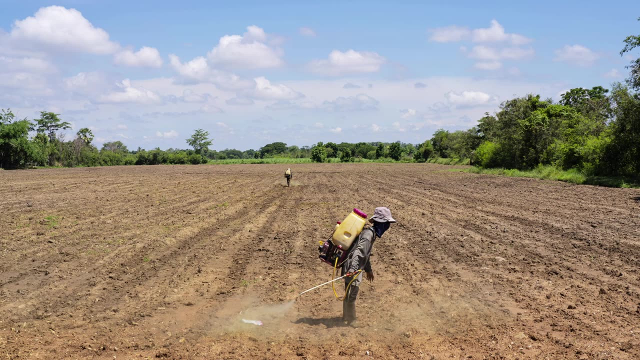 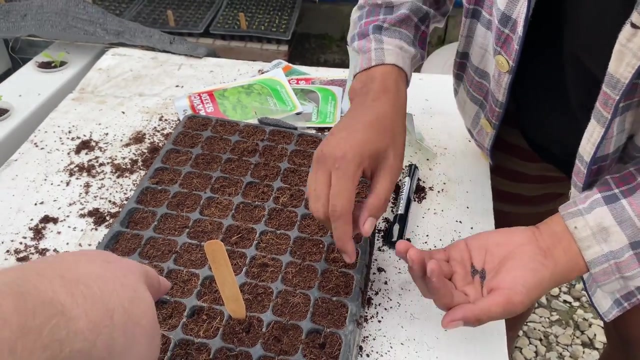 leaves and fruit. Once any of these biotics take hold in your farm or garden, it is very difficult to eradicate other than by spraying herbicides and or pesticides. Many commercial soil-based farms pre-treat the soil with herbicides as a prevention measure. Many of us in hydroponics use cocoa peat or cocoa coir. 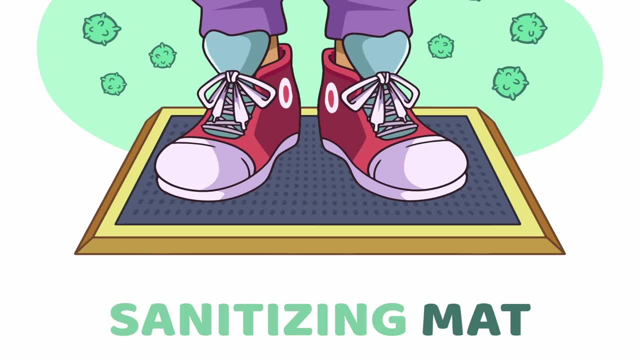 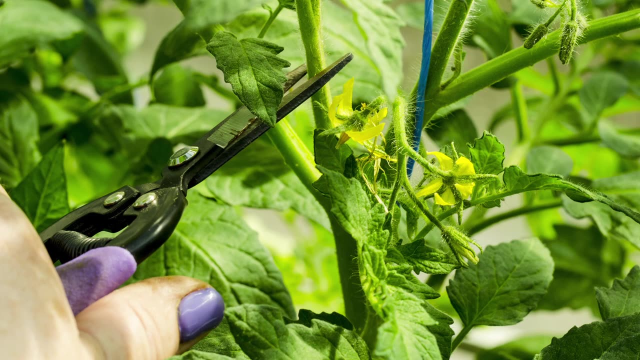 I encourage you to do as we do and boil all the cocoa media before using of having an alcohol tray to step in before entering the greenhouse. Another prevention is to clean the pruning shears in bleach or alcohol after removing diseased leaves. Lastly, we refuse to use pesticides in our 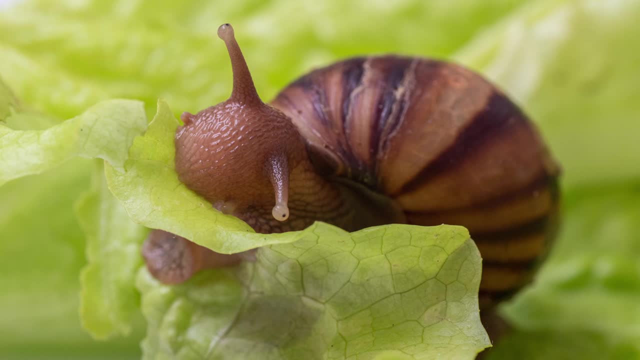 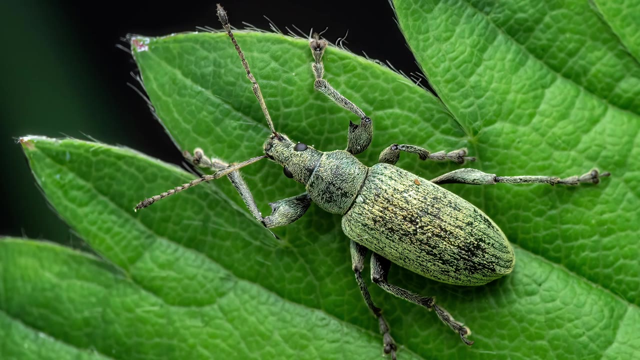 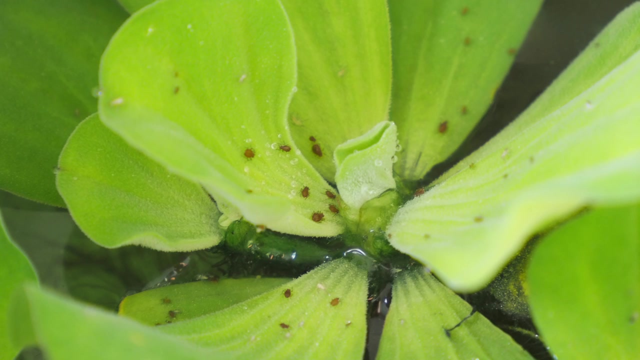 greenhouse. A very effective alternative is to be diligent, and as soon as we see insect damage, it's all hands on deck until we find each and every culprit before they have a chance to multiply. In the case of aphids, there are organic alternatives like spraying the leaves with soapy water. This traps and 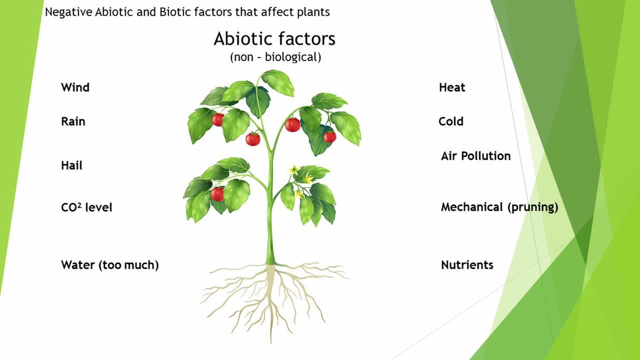 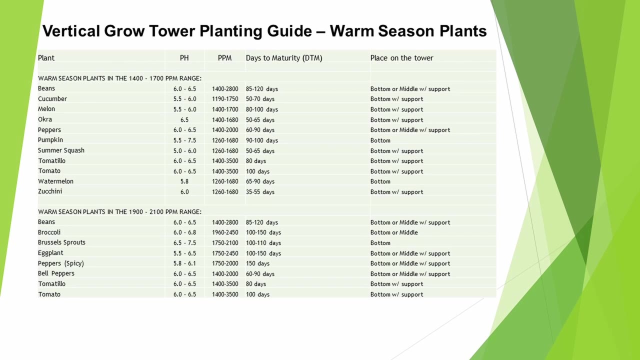 suffocates the aphids. Now on to abiotic factors. We will focus on nutrients In hydroponics. starting with a well-balanced nutrient solution that meets your plants needs is essential, Whether soil-based gardening or hydroponics. know the plants requirements and fertilize accordingly. 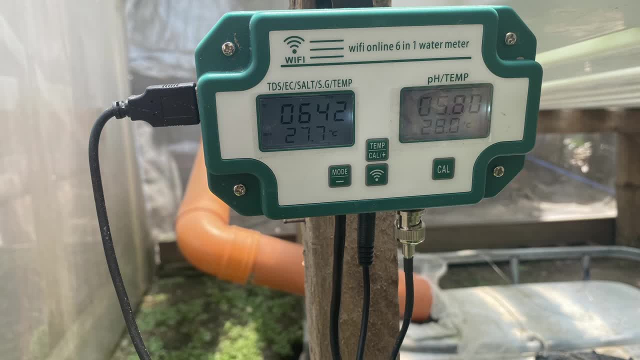 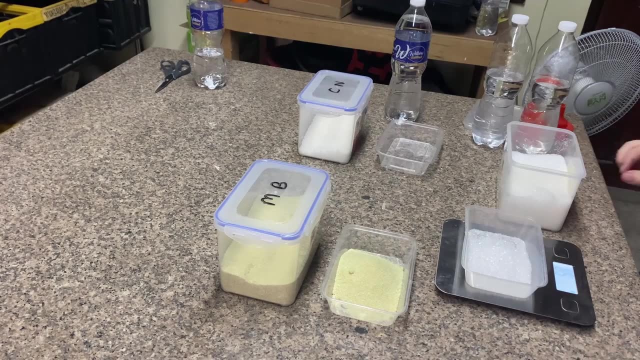 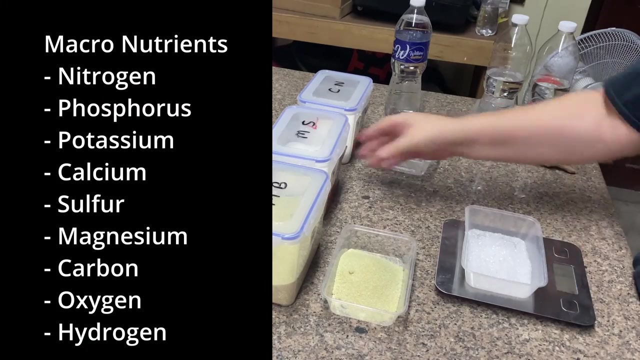 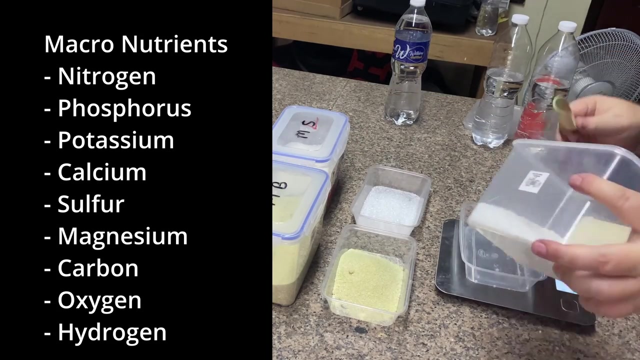 In hydroponics, keep the nutrient solution in the recommended concentration range or PPM level. Nutrients and fertilizers are typically divided into two categories. First are the macronutrients. They are nitrogen, phosphorus, potassium, calcium, sulfur, magnesium, carbon, oxygen and hydrogen. The last three of these are easy. Carbon, oxygen and hydrogen are all provided naturally from aphids and aphids are from aphids. The most common types of aphids are from the air and water, Carbon dioxide and H2O. The first three on the list should 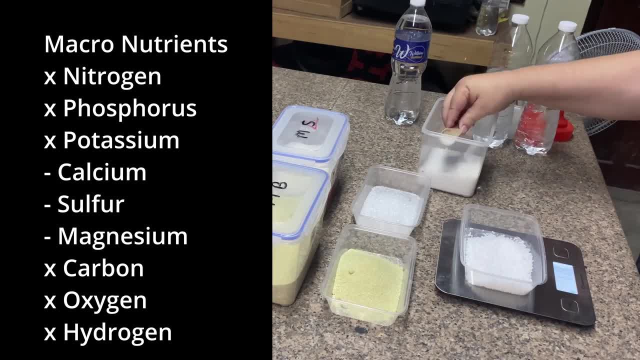 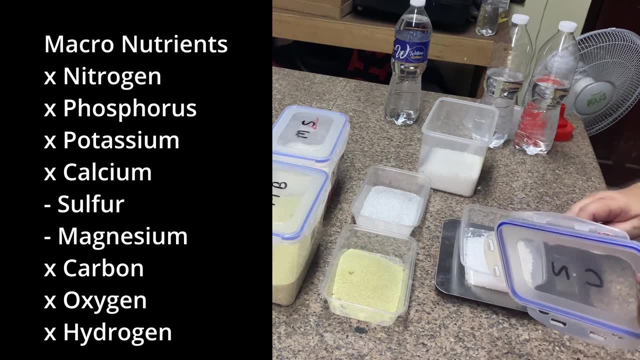 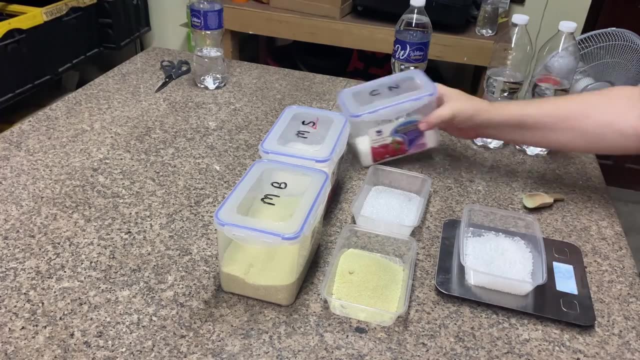 be in the description of your fertilizer: NPK or nitrogen, phosphorus and potassium. Calcium and additional nitrogen are normally added in the form of calcium nitrate. Magnesium and sulfur are added in the form of magnesium sulfate, also called Epsom salt. Micronutrients are also important. They are just needed in. 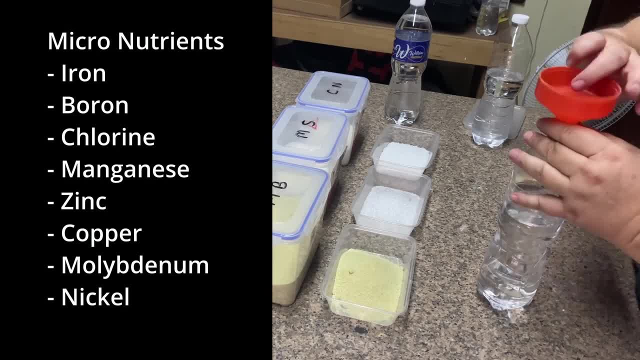 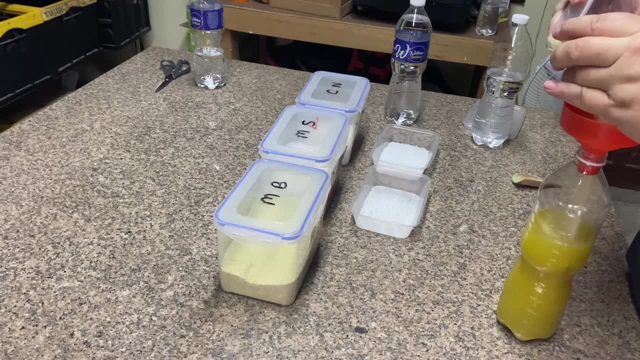 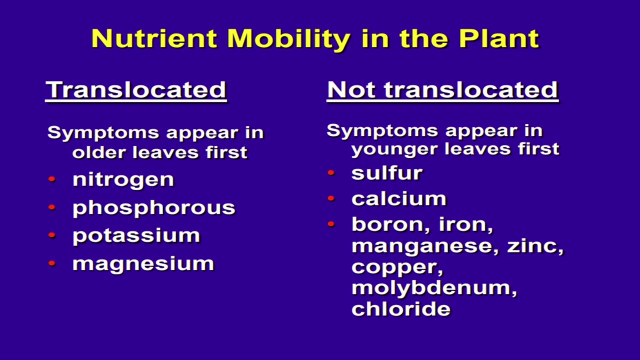 smaller quantities. These are iron, boron, chlorine, manganese, zinc, copper, molybdenum and nickel For hydroponics. these micronutrients should be part of your fertilizer or a solution. Before we go to deficiencies, it is important to 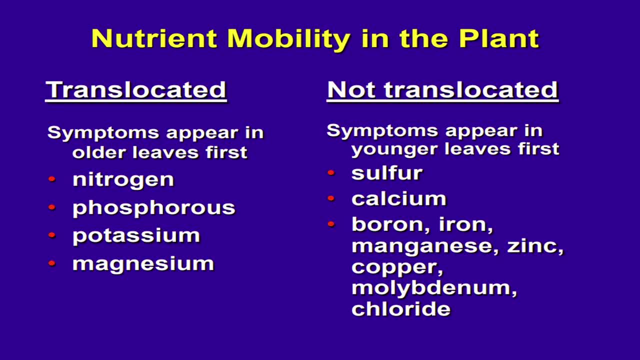 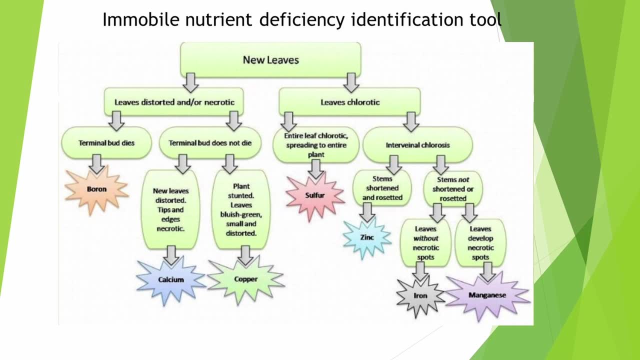 understand that some of these nutrients are mobile and others are immobile. Most nutrients are mobile, meaning that the plants can move these nutrients from older tissue to newer tissues. Immobile nutrients cannot be moved to new or tissues. This is helpful in identifying the nutrient deficiency. 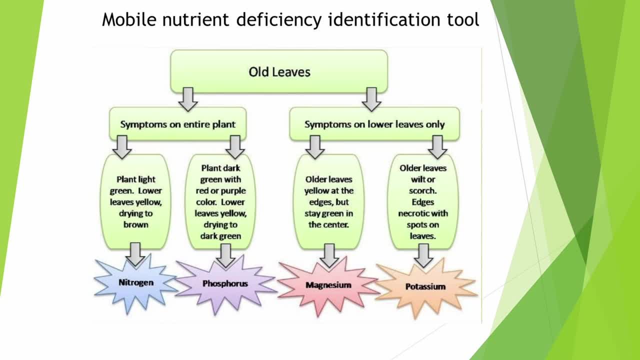 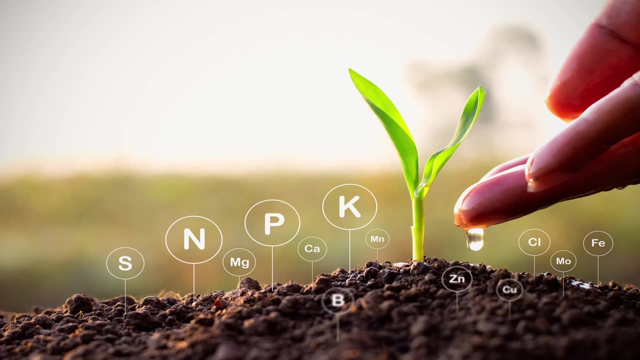 Deficiencies of immobile nutrients will show evidence only in the younger growth and new leaves, Whereas deficiencies in mobile nutrients will show on the entire plant. Calcium, sulfur, iron, boron and copper are all immobile nutrients. Let's focus on the more common nutrient deficiencies, starting with the mobile. 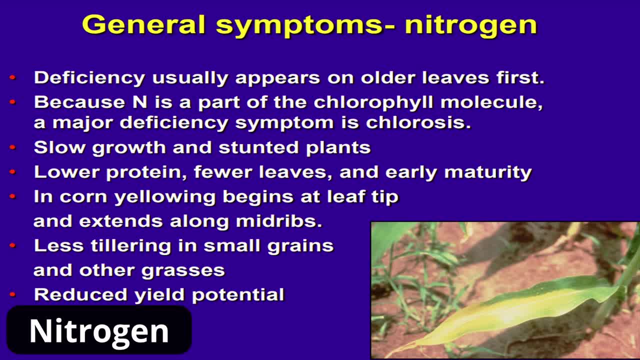 nutrients and how to recognize them. Nitrogen is needed by plants to produce nutrients. Nitrogen is needed by plants to produce nutrients. Nitrogen is needed by plants to produce nutrients. Nitrogen is needed by plants to promote rapid growth, especially for fruit and seed development Also, it 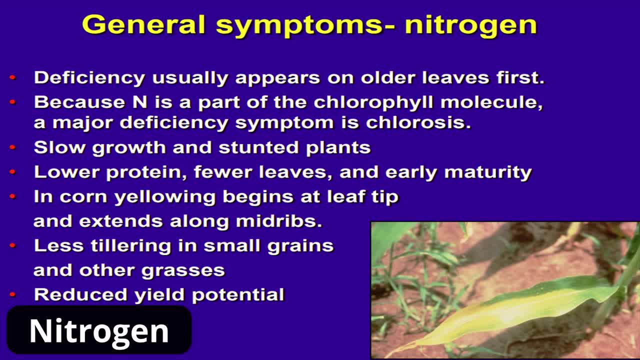 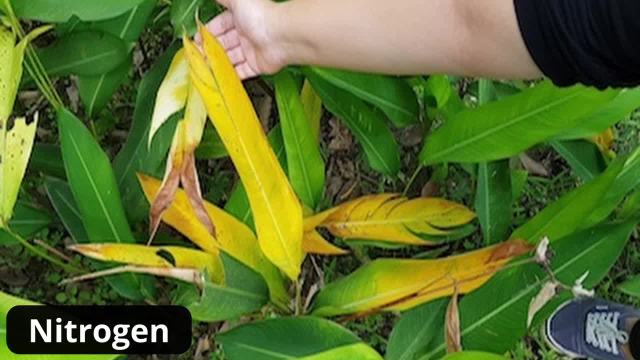 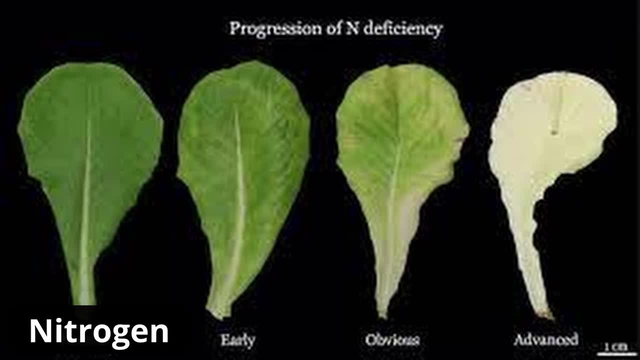 increases leaf size and quality and hastens plant maturity. Deficiency symptoms are the changing of the entire plant to a light green, followed by yellowing of older leaves proceeding towards younger leaves. Plants become spindly, stunted and secondary shoots develop poorly. if the initial symptoms 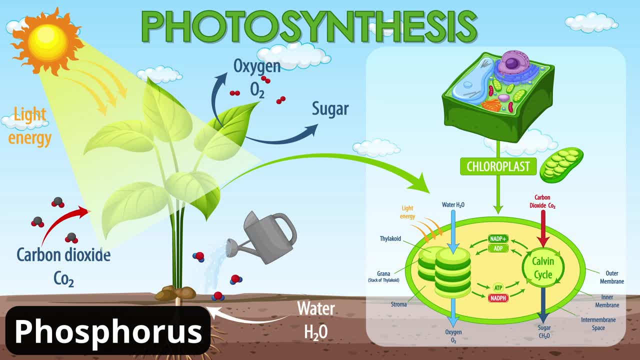 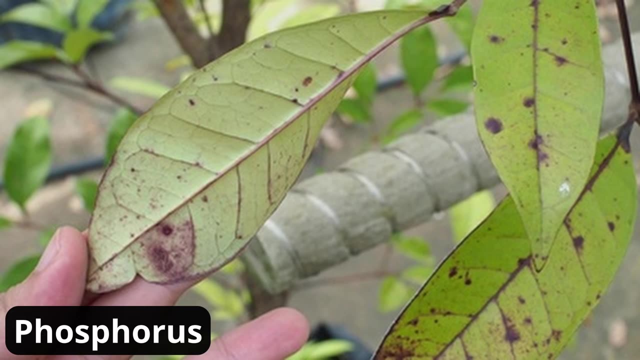 are not corrected. Phosphorus is needed by plants to promote photosynthesis, protein formation, seed germination, bloom stimulation and budding. It also hastens maturity Deficiency symptoms are purple or bronze coloration to the underside of older leaves. Effective plants develop very slowly and are stunted compared to 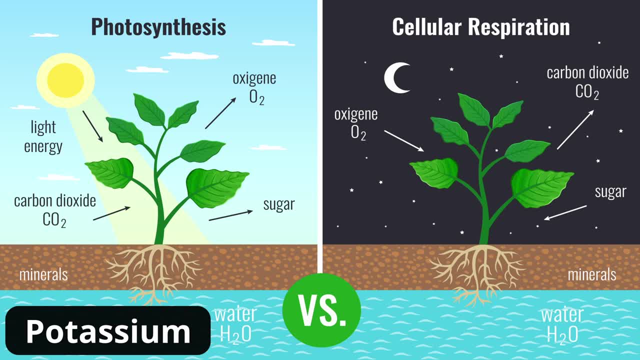 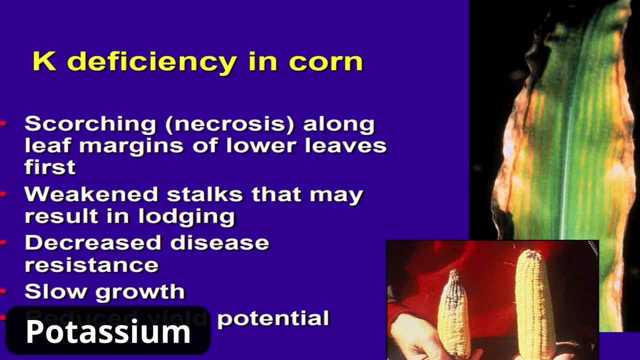 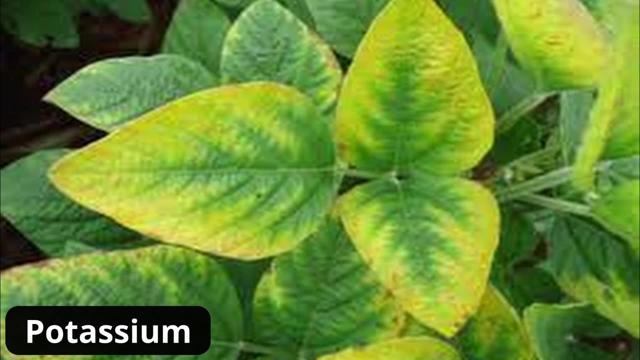 normal plants. Potassium is needed by the plants to promote formation of sugars, for protein synthesis, cell division in plants and for root development. It also increases the plant's resistance to diseases. Deficiency symptoms are leaf edge yellowing on mature leaves, followed by intravenal scorching and necrosis from. 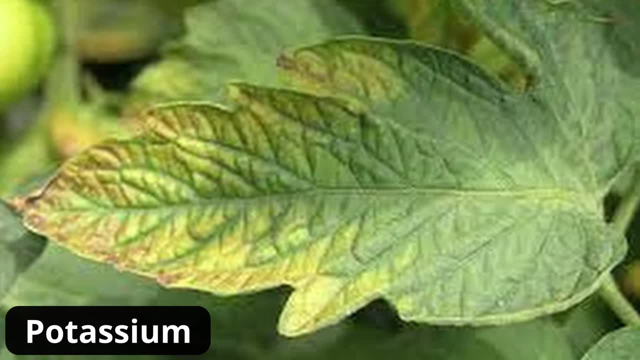 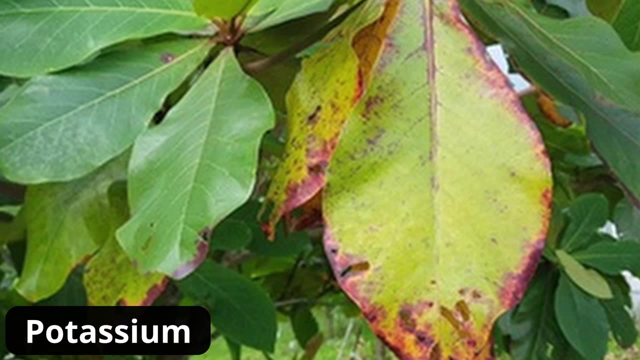 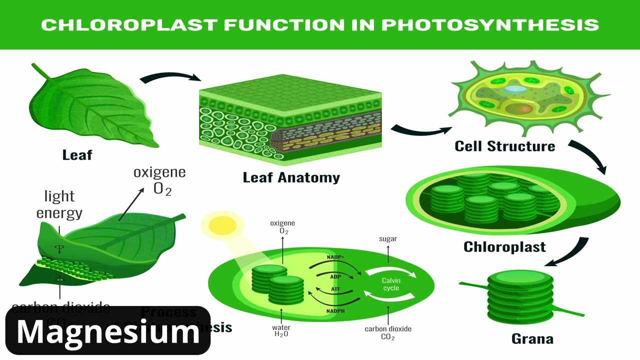 leaf edge to the midrib as deficiency increases. Potassium deficiency is irreversible. Even if potassium is given to the plants, the leaves will not recover. Magnesium is needed by plants to promote the function of plant enzymes to produce carbohydrates, sugars and fiber. Potassium is needed by plants to promote the function of plant enzymes to produce carbohydrates, sugars and. 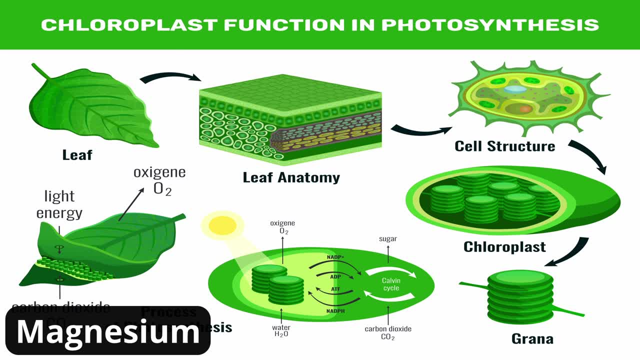 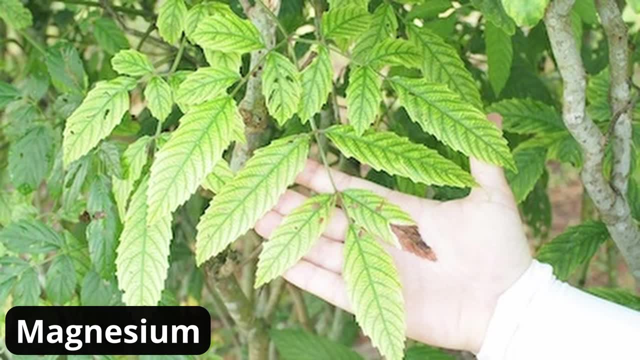 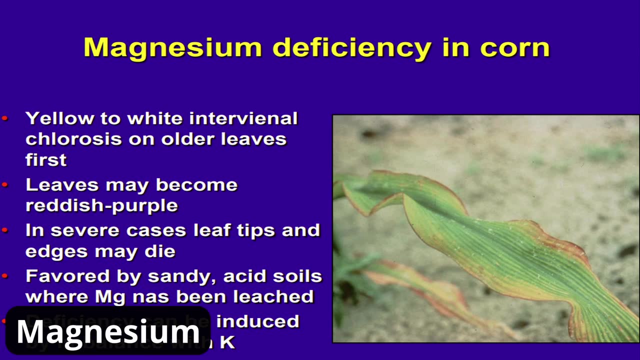 fats and in the regulation of nutrient absorption Deficiency. symptoms are older. leaves will lighten or yellow. between veins This is known as intravenal chlorosis. In severe deficiency, plant growth rate drops, leaf size is reduced and lower leaves are shed. Now on to the common immobile nutrient deficiencies. 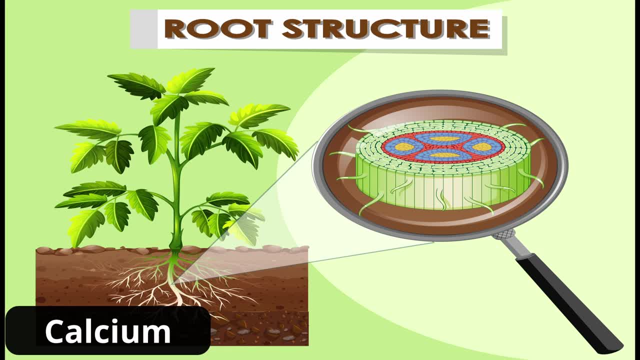 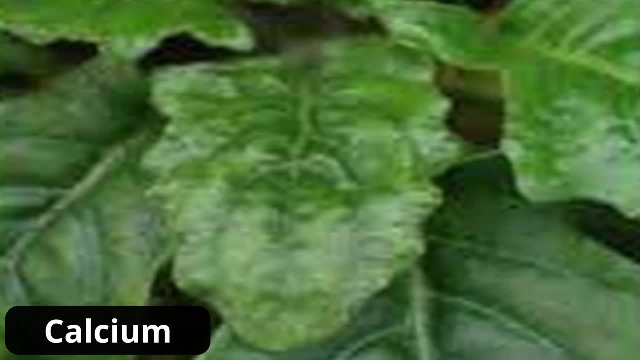 Calcium is needed by plants to produce new growth and root tips. Calcium is a nutrient that is immobile. Other action that is needed is to take calcium from plants to produce new growth and root tips. Calcium is a nutrient that is immobile within plants. The first symptoms will show on new leaves and leaf tips. 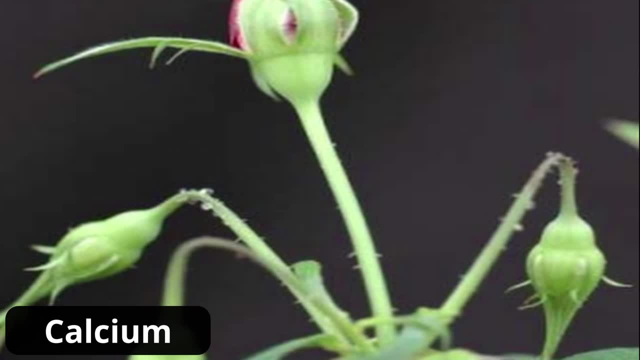 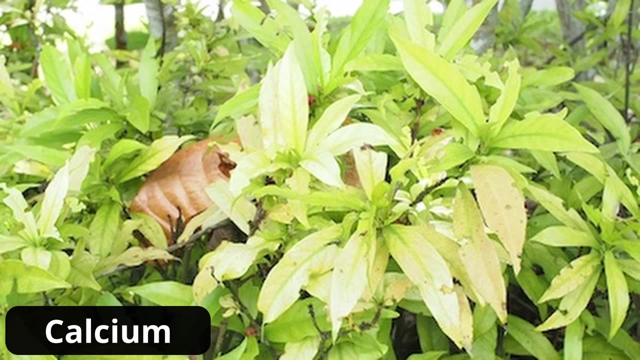 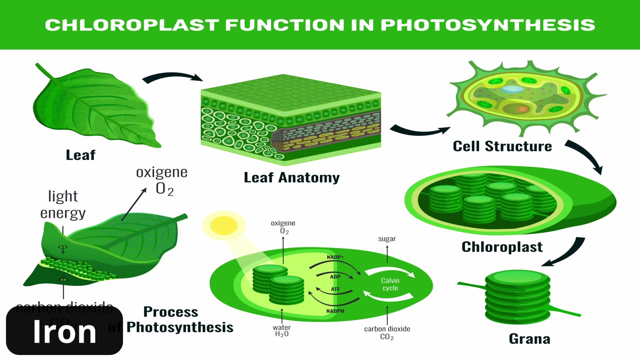 Deficiency symptoms are: new foliage buds and roots have stunted growth. Younger leaves curl downwards with browning of leaf edges and leaf tips, also known as tip burn. In some plants they may also show abnormal green foliage Roots become short and stubby. Iron is needed by plants for the synthesis of chloroplast. 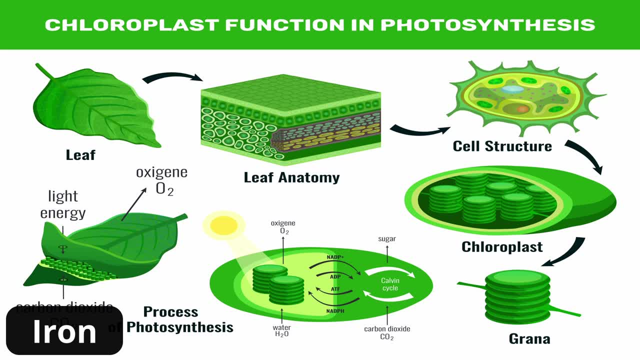 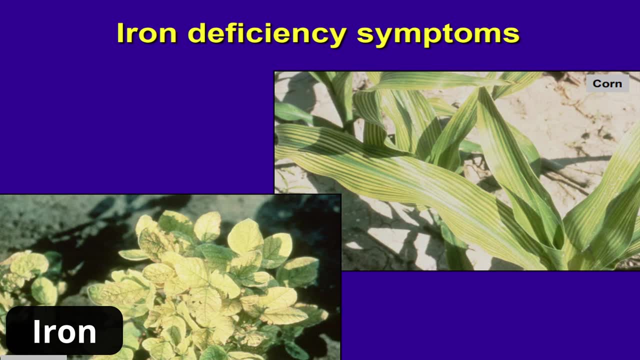 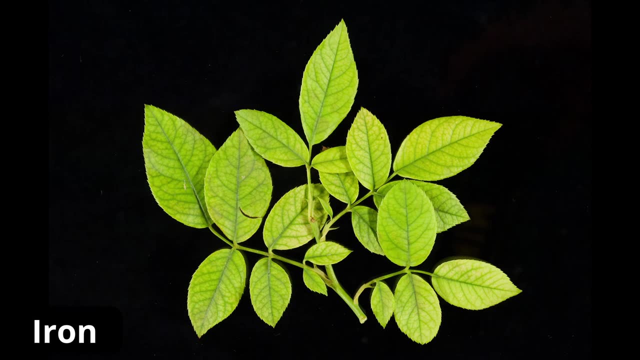 proteins and various enzymes. Iron deficiency is similar to magnesium, except since it is an immobile nutrient. the evidence will show on the young leaves and leaf tips. Deficiency symptoms are light green to yellow interveinal coloring on new emerging leaves and young shoots. It is common to 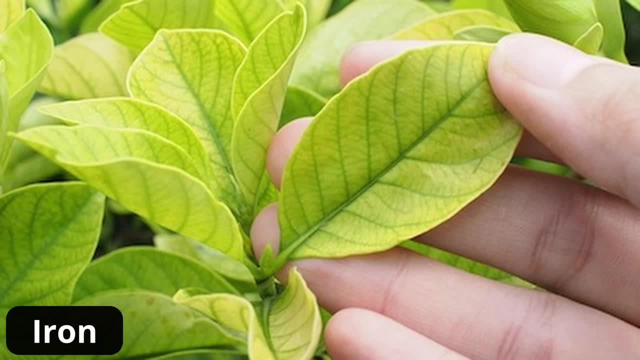 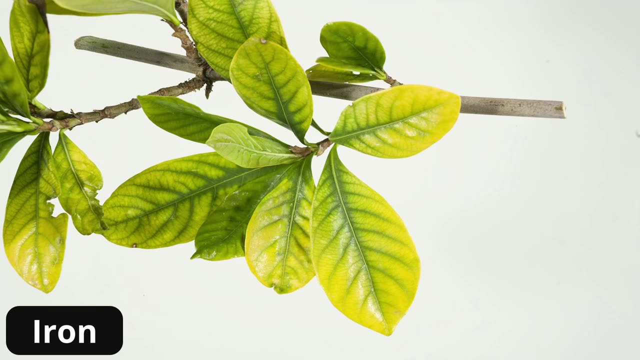 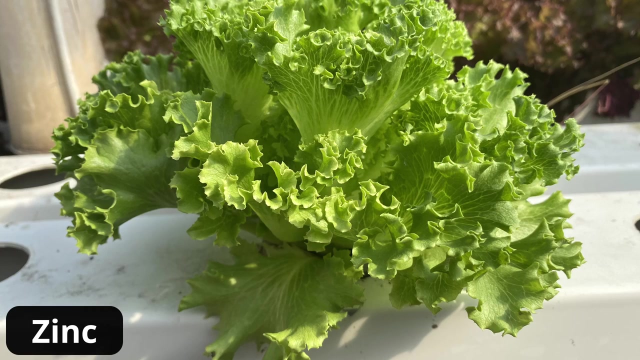 see shoots dying from the tip inwards. In severe cases, newly emerging leaves may reduce in size and turn nearly white With necrotic spots. zinc is needed to activate plant growth regulators. Deficiency symptoms are yellowing, bronzing or modeling of younger leaves. 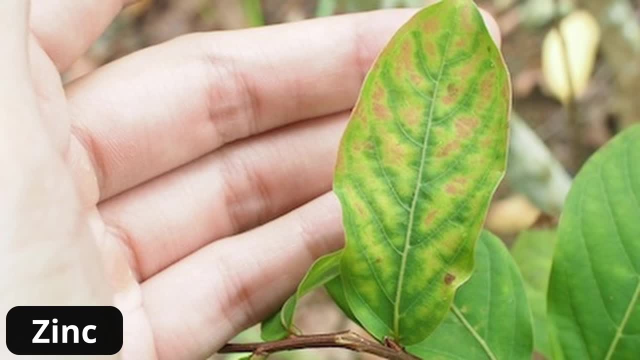 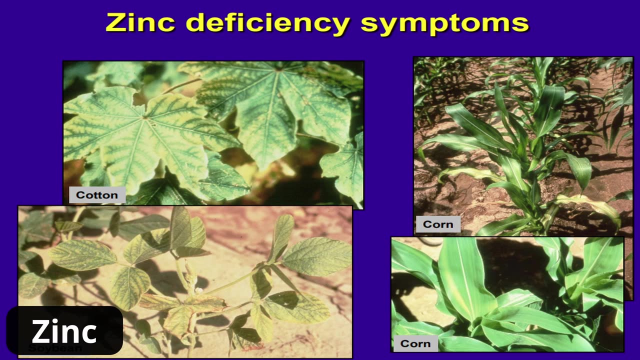 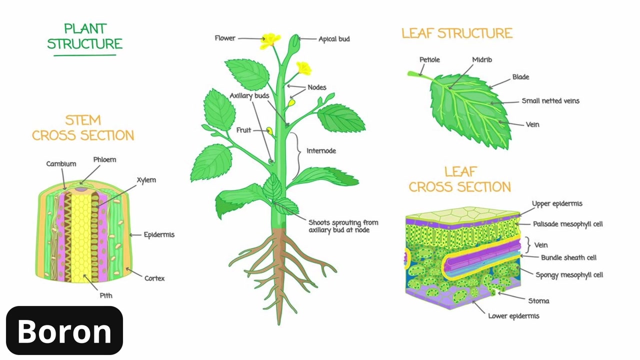 Interveinal yellowing of the young leaves, followed by reduced shoot growth, as well as small and discolored leaves, giving the affected part a rosette appearance. Boron is needed in the process of cell differentiation at the growth tips of plants where cell division is active.